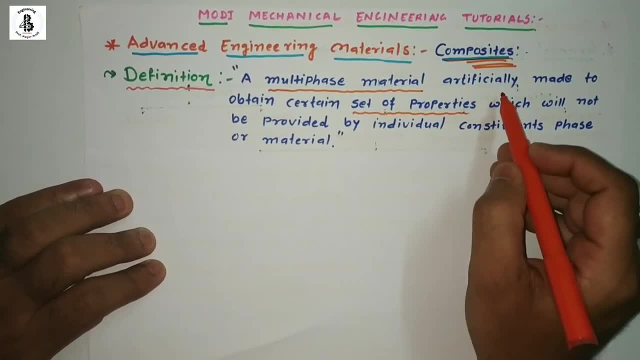 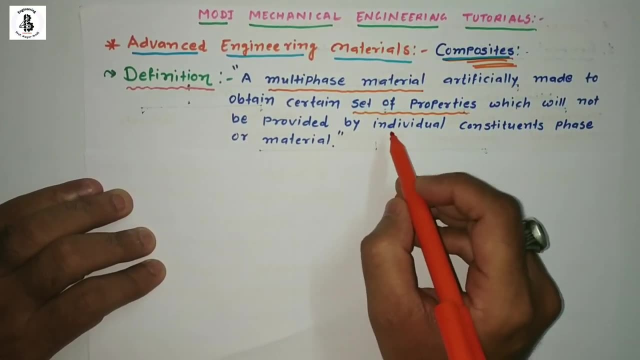 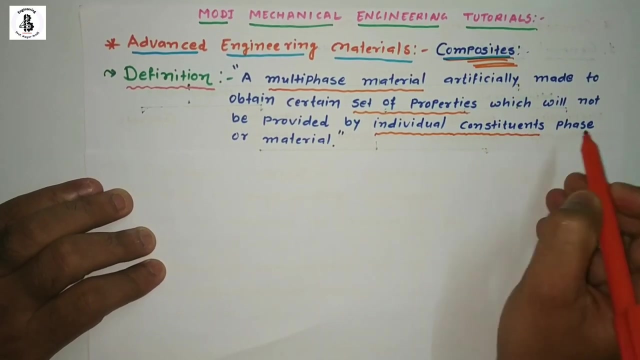 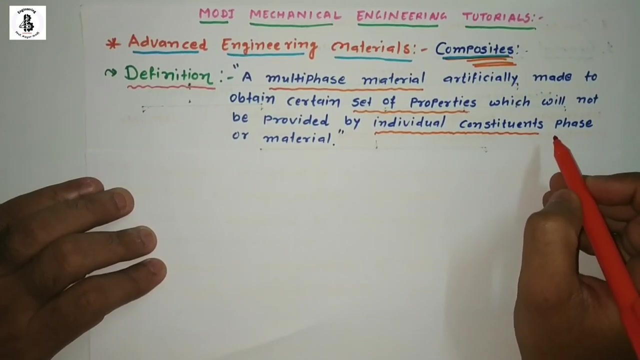 So here a multi-phase material, artificially made to obtain the certain set of the properties which will not be provided by any individual constituent, or you can say it will be not fulfill all the kind of satisfactory results As a single metallic constituent. So then it will be make of multi-phase materials. 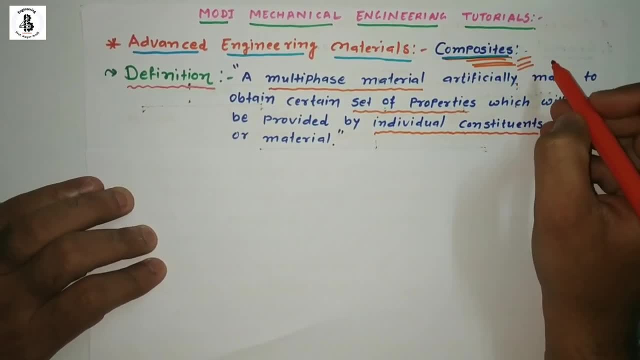 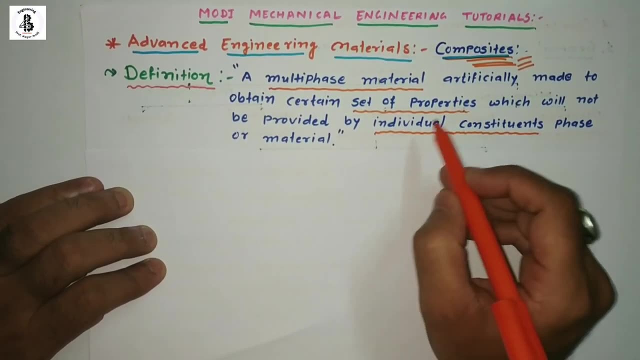 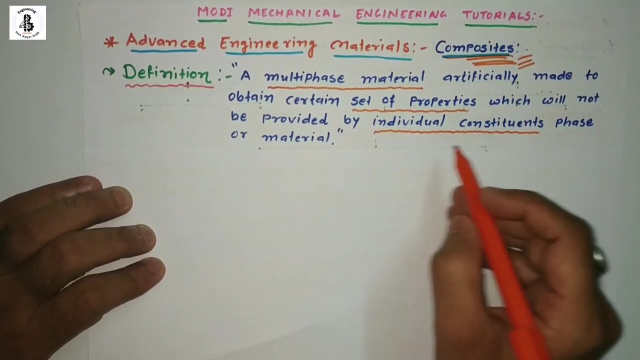 So that would be called as a composite materials. So basically that would be artificially addition of the two materials which will be having a good set of the properties to be training, such under the loading condition of the product. So it would be called as a composite materials. 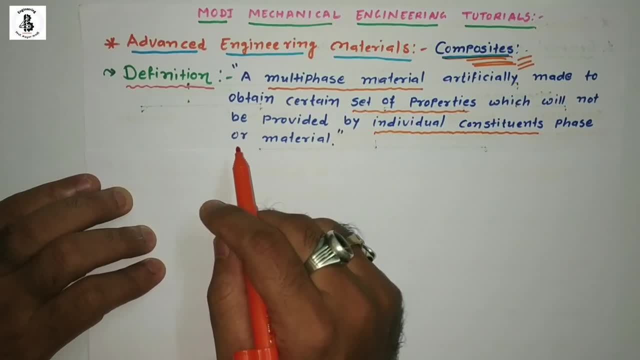 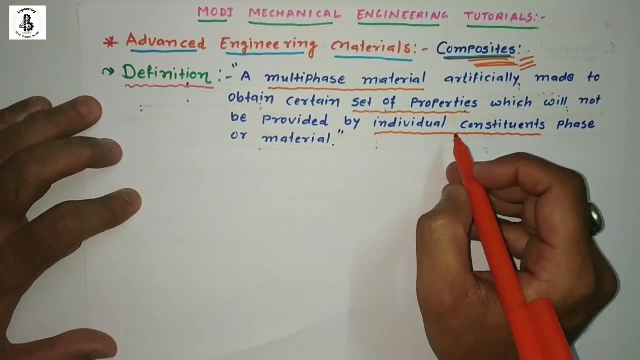 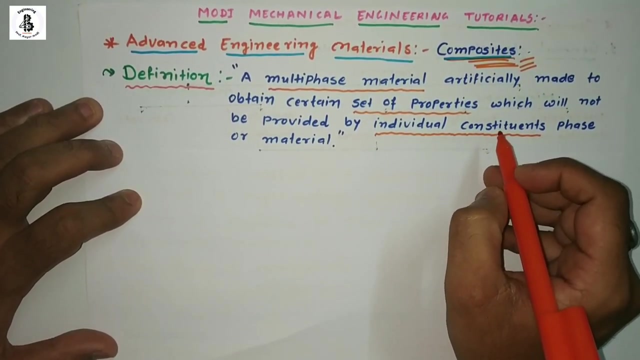 So nowadays, all the industries that will be focusing on to that particular advanced material which will be having a good performance with the minimum cost of the manufacturing, as well as the raw materials, and that will be having a low density material, So low weight material, it will be having a higher specifications to performing all the under the 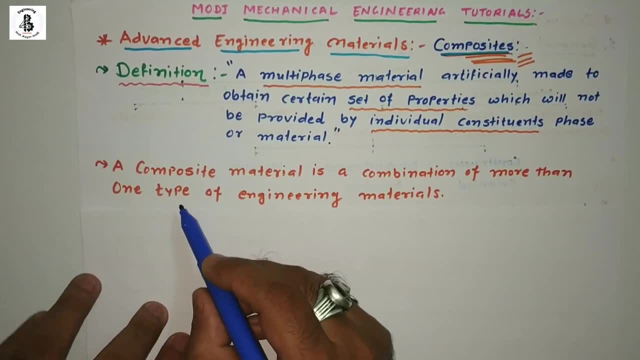 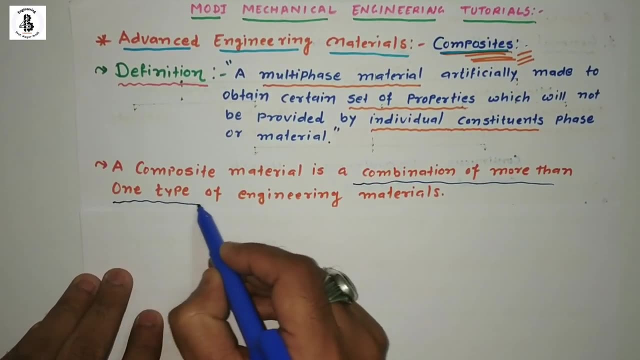 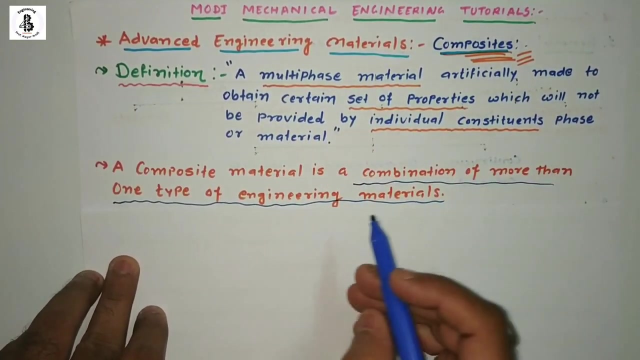 conditions of the product. So a composite material is a combination of more than one type of engineering materials. So that will be from the definition wise, it will be the multi-phase materials. So more than one type of engineering materials is being used for developing that. 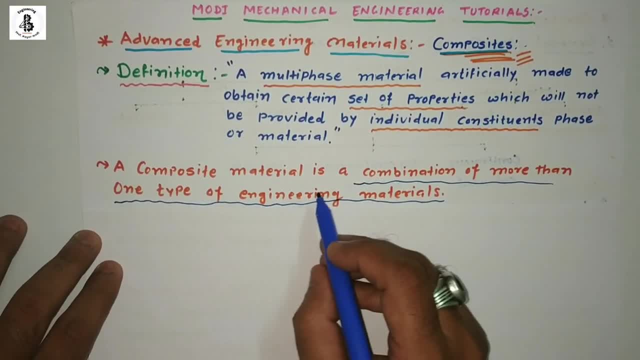 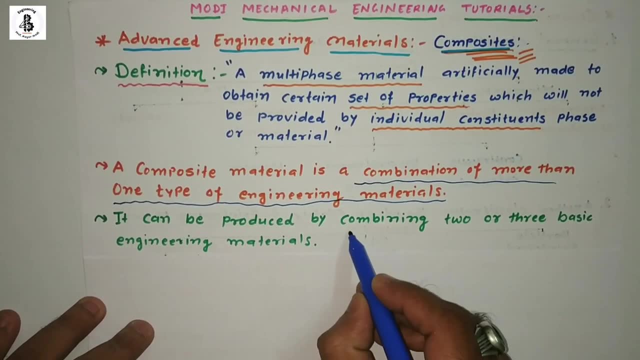 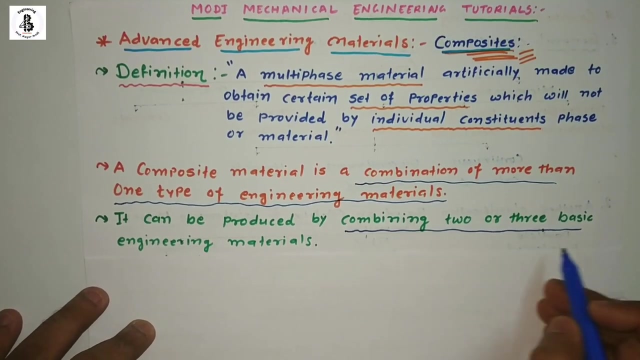 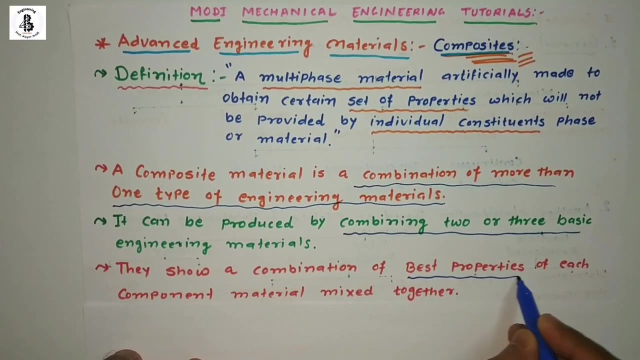 multi-phase material which will be having a higher specifications as compared to the individual constituents. So it can be produced by combining two or more basic engineering materials to form a composite material. So that will be from the definition. wise, it will be the composite materials. They show a combination of the based properties of the each components. 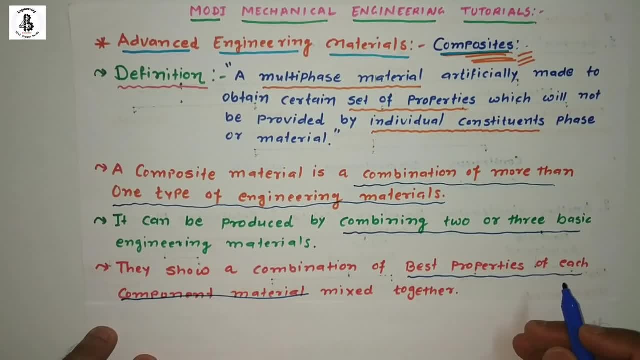 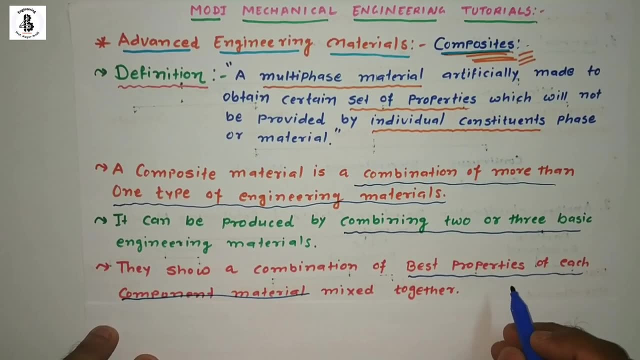 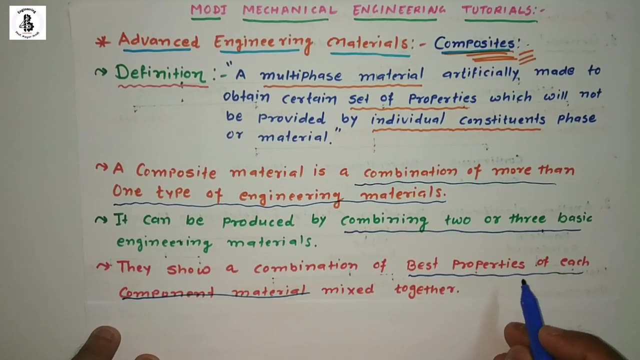 of the materials mixed together and to form the new materials. So generally it will be- only depends upon the engineering requirements of the material. as from the applications- So applications- it going to be changed. its properties is being changed, So that will be from the definition. wise it will be. 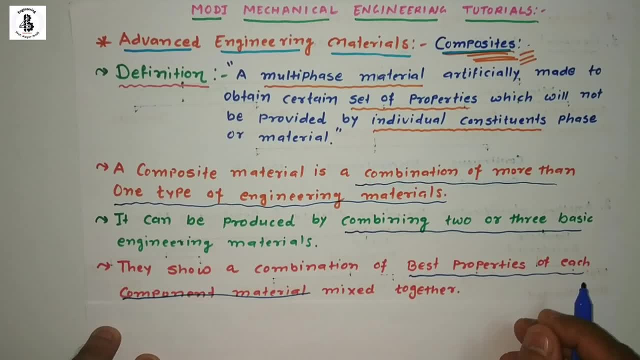 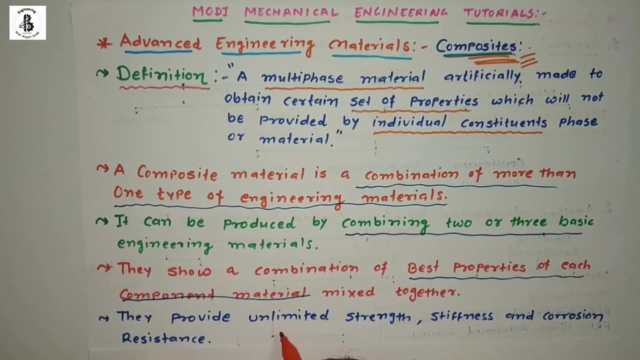 being changed and the selection of the materials is also changed. For the selection criteria I already made one video So you will find a link in my description box. So by the addition of the two or three basic engineering materials, so they provide ultimate strength. So that will be from the 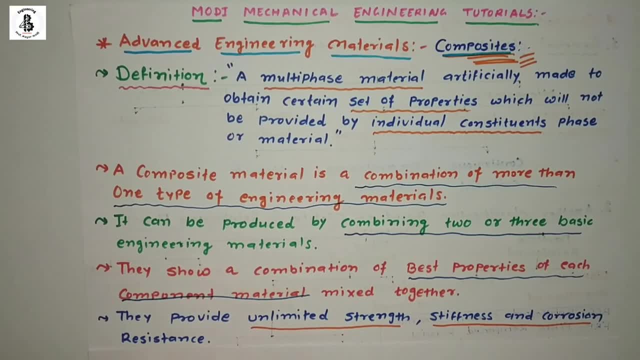 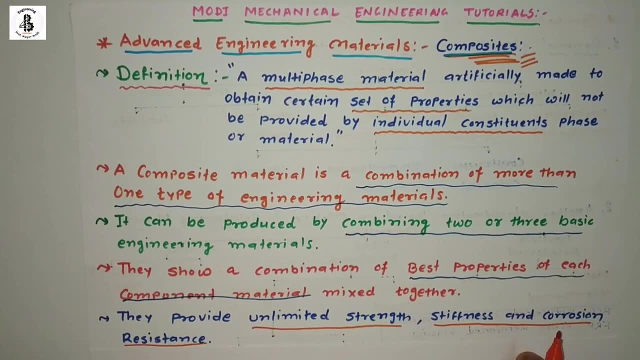 mechanical stiffness and the corrosion resistance. So such kind of properties it will be present. or you can say such kind of mixed properties. So that will be from the definition wise, it will be present, or it will be present into the materials And nowadays, into the advanced engineering. 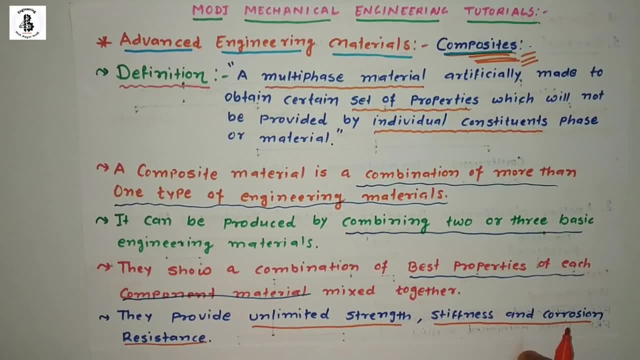 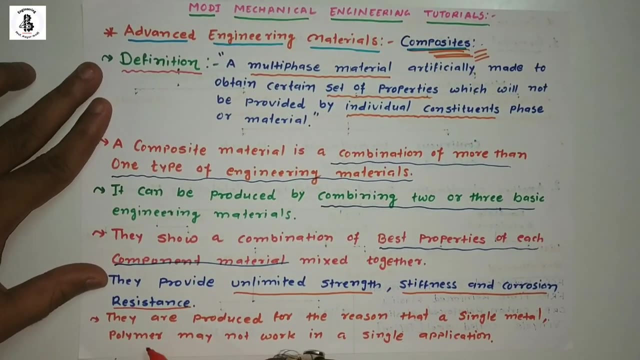 materials that all are the requirements. Low weight, high specified materials is being required for the aerospace, military and mining industry. So there are so many advancement with the engine as a composite material. So they are produced for the reason that a single metal polymer may not be. 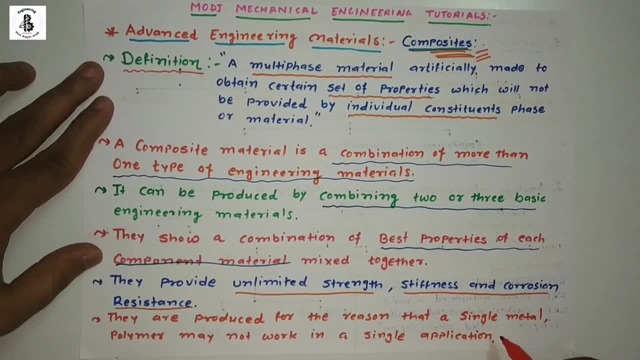 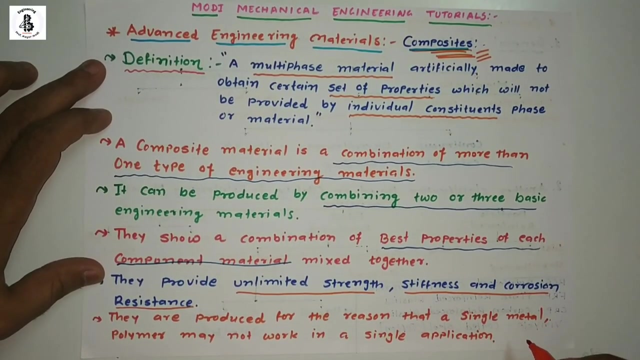 in a single applications. so as per the requirements of the materials for the engineering applications, so single metallic materials, it will be not appropriate to work under the heavy loading conditions. so that will be the best option for the engineering advanced material as a composite materials. so most of the product now it will be replacing by the composite materials. so that will. 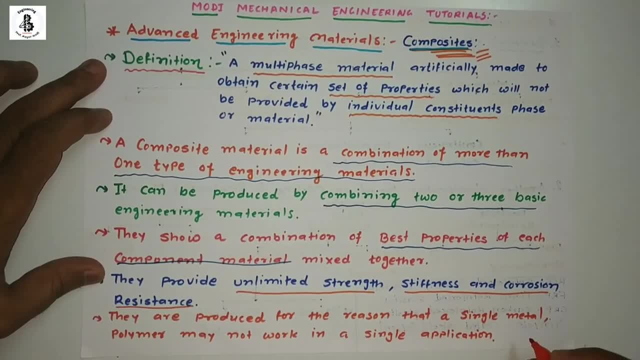 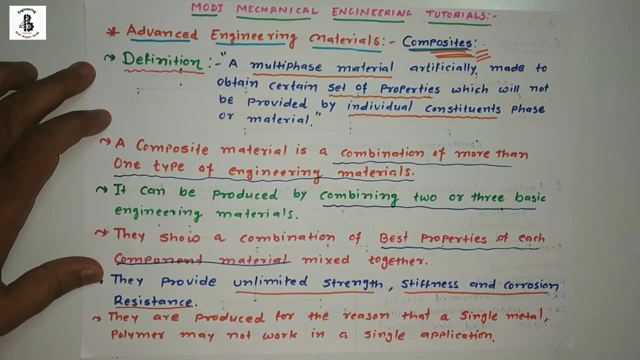 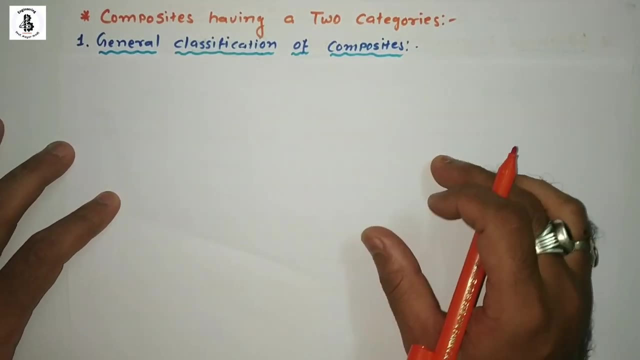 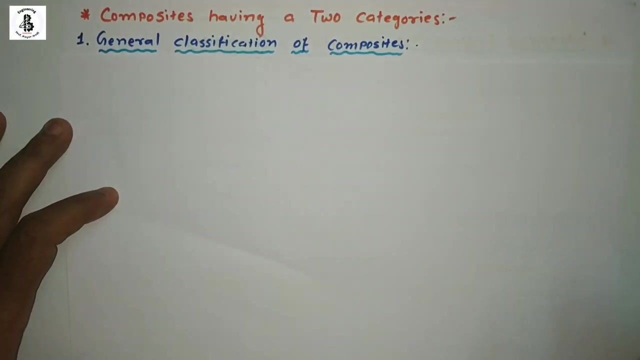 be having a good economical consideration. it will be having a good fabrication facility as well as it will be having excellent service conditions. that will be the most focus area for selection of the advanced engineering materials. now we will discussing with the composite, having basically two categories now: first, discussing with the general classification of the composite, if you. 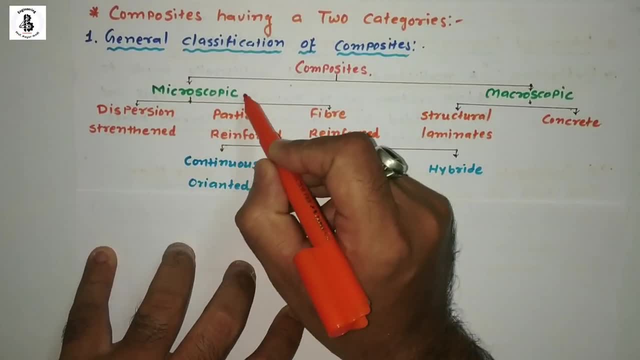 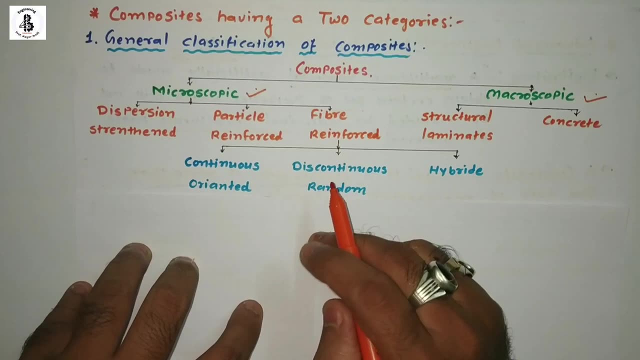 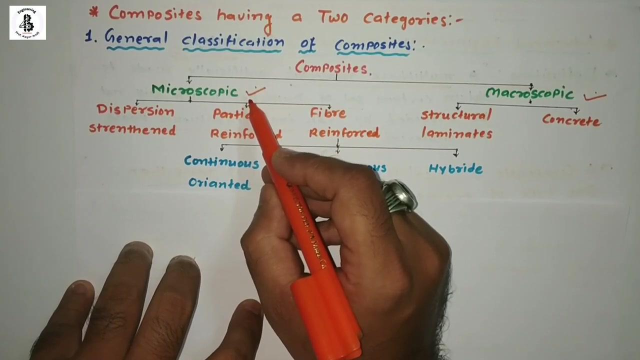 observed a composite materials at microsoft microscopic level and macroscopic level. basically that will be the two kind of levels of the testings of the metallic materials. so at microscopic levels and you can see that more than 16 x of the zooming facility it will be available for the testings and for the macroscopic. so in the case, 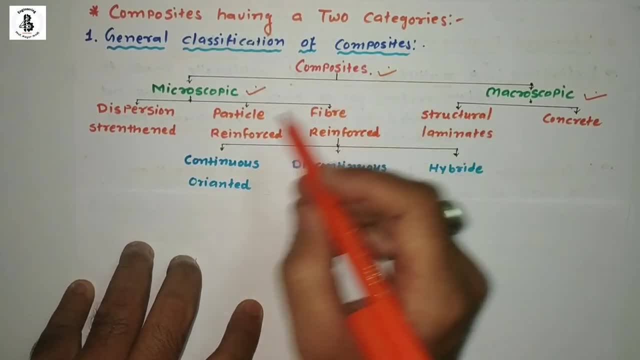 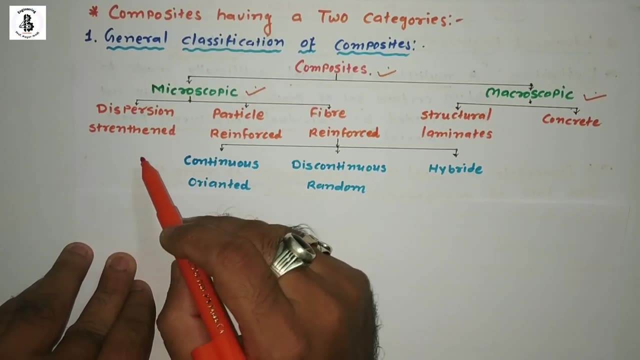 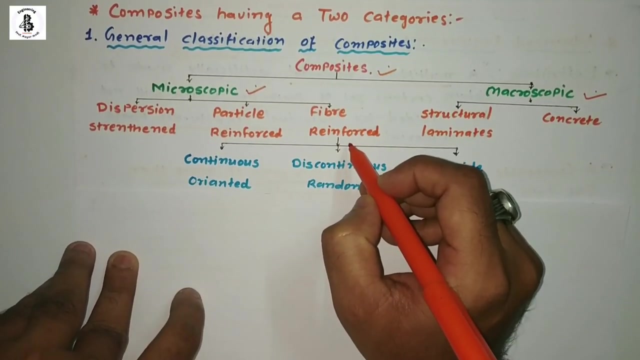 of the microscopic examination of composite materials first, according to the orientations of that structural part of composite, it will be having a good classification of the composite materials and these types of testings will be having a dispersion strengthen particle, this reinforced and fiber rain form. so basically, in the case of the dispersions, both the, both metals. 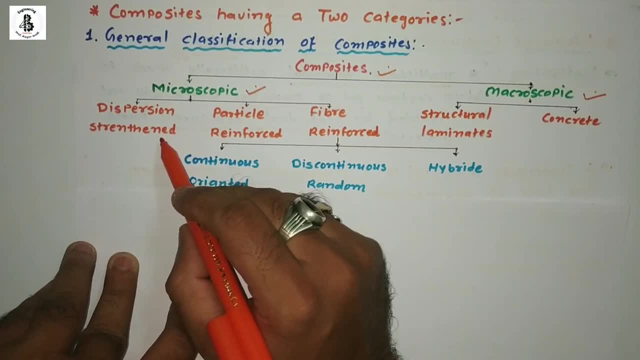 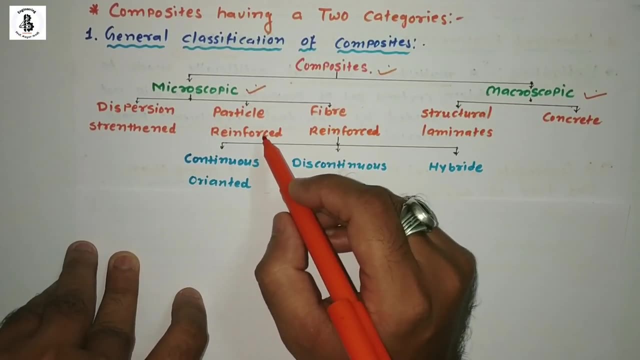 one can say selected materials. it will be easily. dispersion strengthening is cited into the ¬MICROSCOPIC LEVEL particle reinforced, so some hot particles. it will be introduced into the basic metallic structure so you will easily find this particle can be ہیں analyzed in a draining method and in this way in practice you can told that is a Reforgedhack tamam. so you could look at the toner both of the Iowa vs W Kolleginnen materials. deluxe residence level noise in terms of heart particles and the same way this did not become a compound. it now have become a subject for the hard expressing coating it will also need about theSorry, the strength of human hard particles. so you 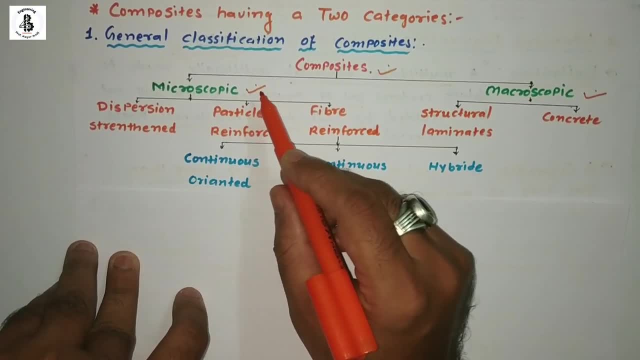 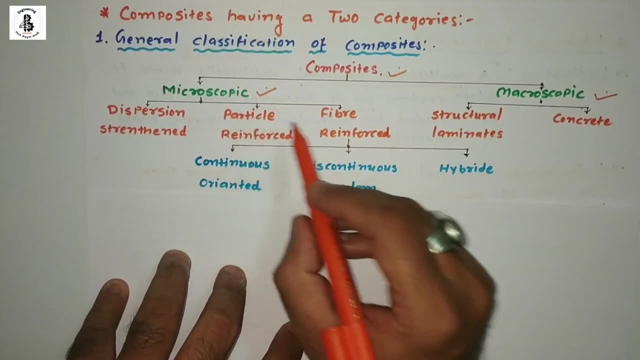 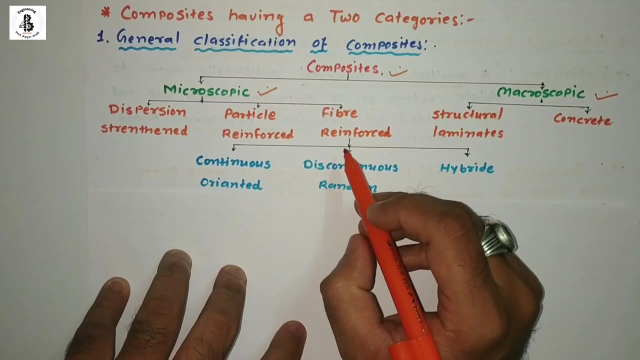 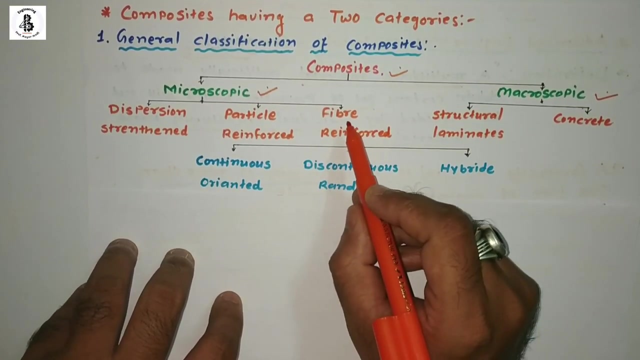 kind of structure. it will be into microscopic level as a reinforced material to form a composite material. then microscopic level, some fibers, it will be oriented into the structure. so that will be considering as a fiber reinforced kind of composite materials. so once again, these fiber reinforced composite materials nowadays it will be having a maximum applications in the field of 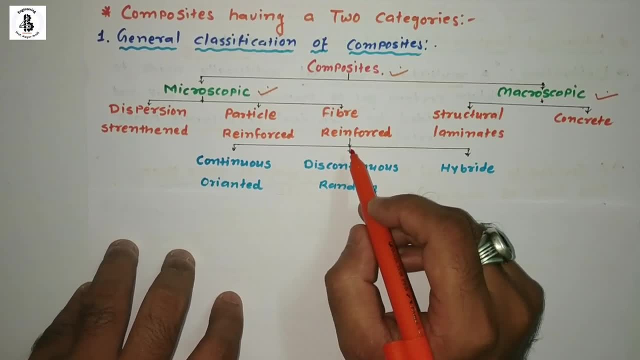 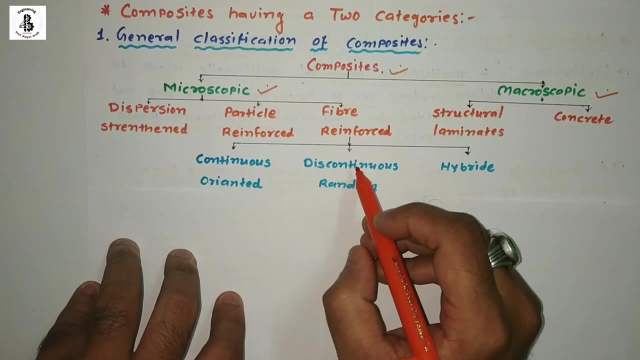 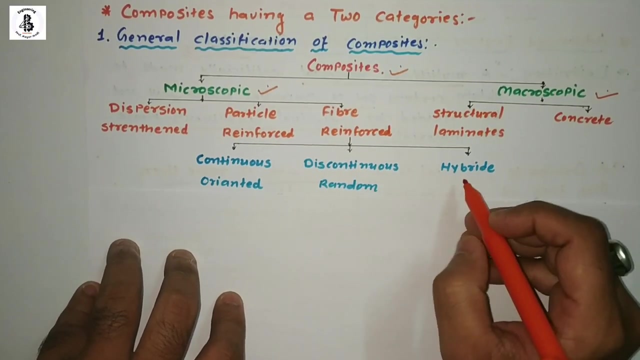 aerospace engineering, mining industries and military applications for basically low weight, high specified metallic materials. so in case of the fiber reinforced material it will be having a continuous orientation, discontinuation kind of orientations, or you can say random orientations of the fiber into the reinforced and hybrid orientations. so basically this orientation you should find at a 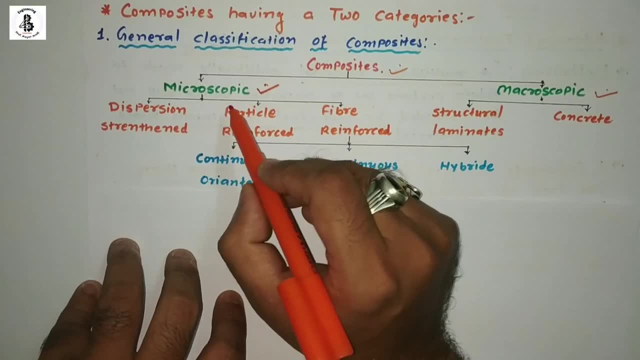 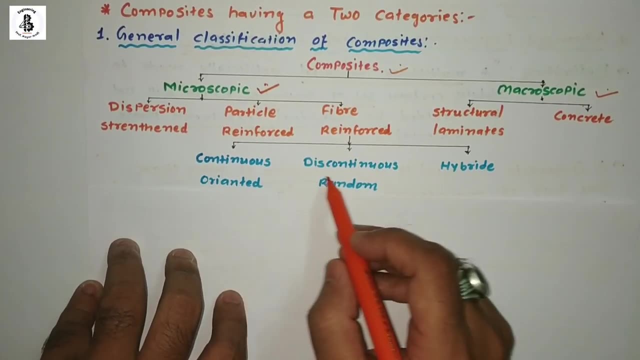 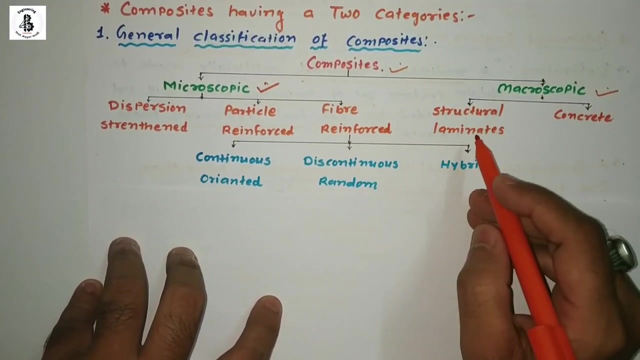 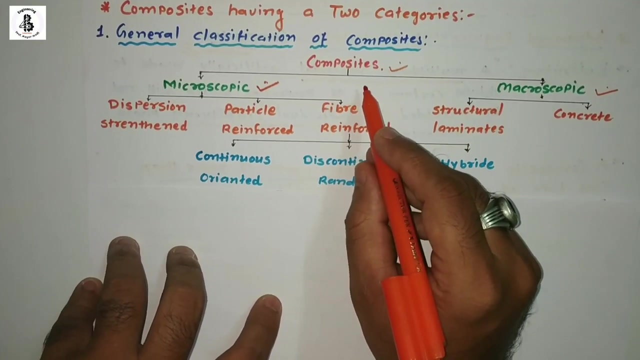 microscopic examinations, so by the applications of microscopic examinations. basically, in the case of fiber reinforced, it will be three category: continuous, discontinuous and hybrid. now for the macroscopic examinations for the composite materials. it will be identified as a structural laminates and concrete kind of structure for the composite materials. so these all are considering as a general classification of 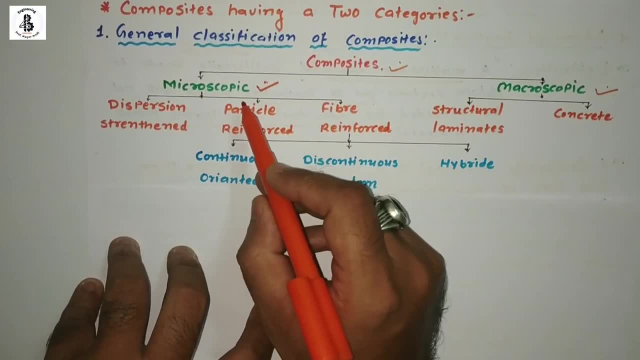 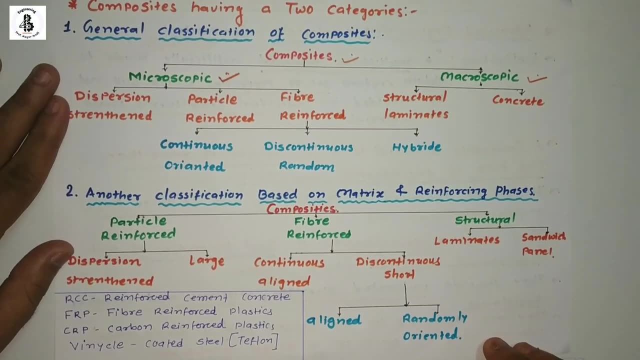 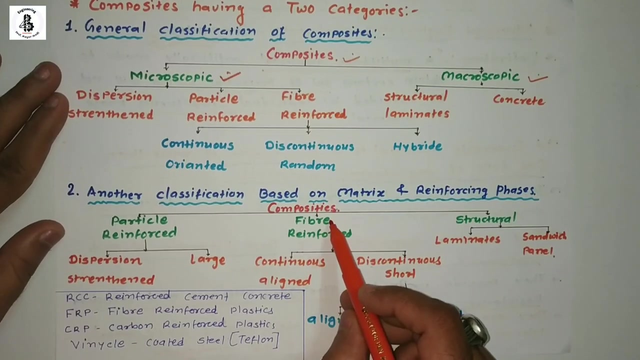 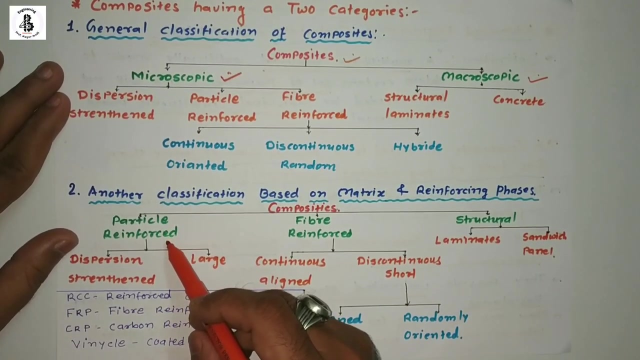 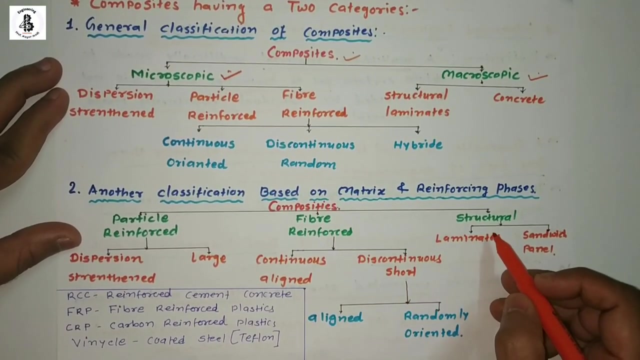 composite material at the microscopic and macroscopic level of the examination. another classification based on a matrix and reinforcing phases, so basically composites, it will be categorized in the case of the matrix and reinforcing phase is a particle reinforcing, so some heart particles. it will be reinforced, fibers reinforced and structural reinforced. so